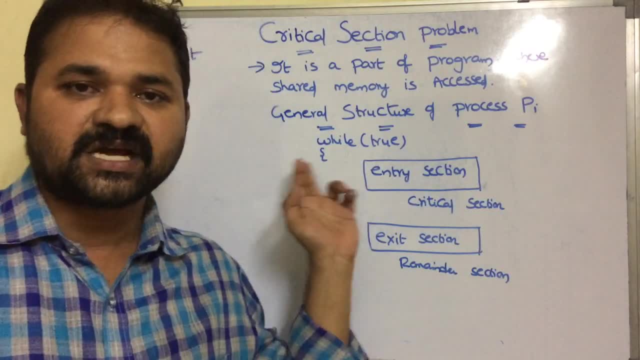 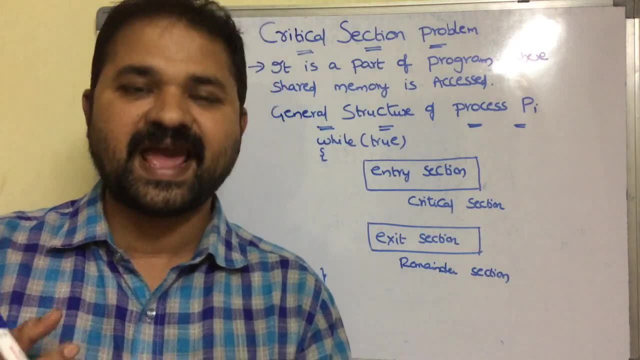 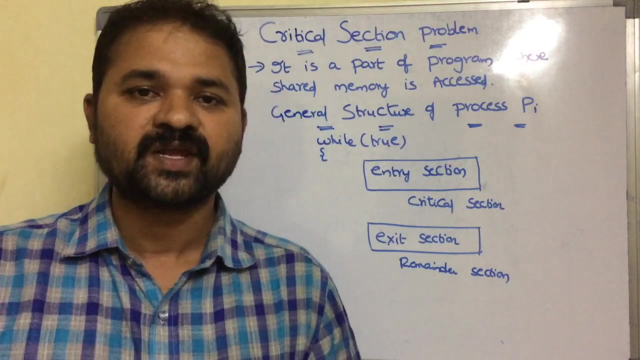 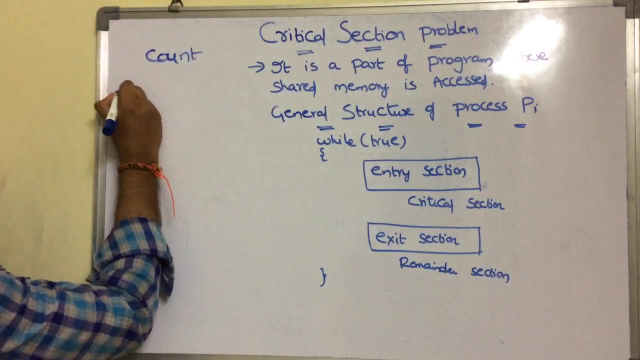 Suppose if the buffer contains only two items, then the count value is two. Suppose if the buffer doesn't contain any items, then the count value is zero. like that In producer consumer problem, the producer process produces an item And the corresponding item will be stored in the buffer and after that the count variable will be incremented by one. 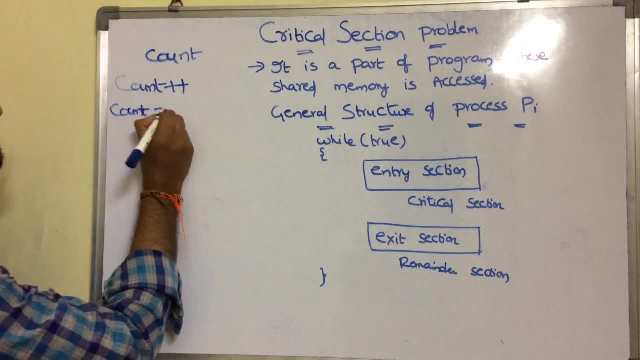 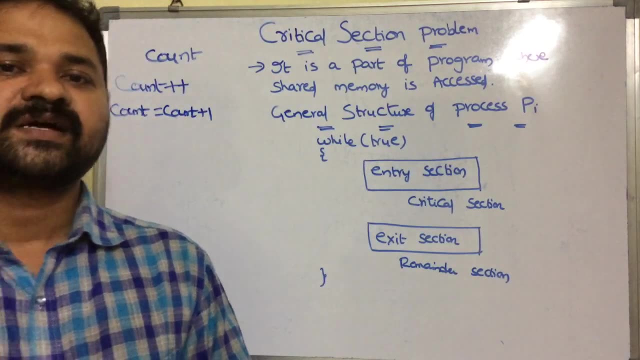 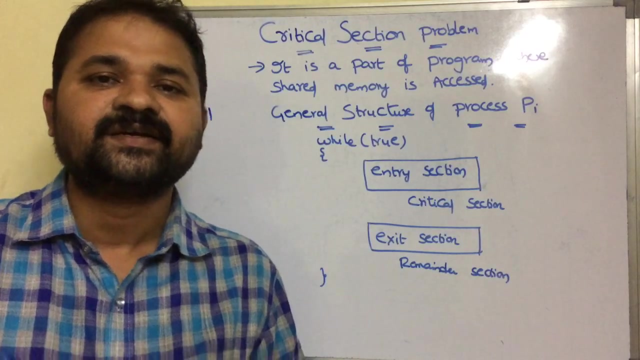 So that is nothing but count++. So count++ can also be written as: count is equal to count++. So in a similar manner, the consumer process consumes an item from the buffer And it decrements the number of items, And it decrements the value of the count by one. 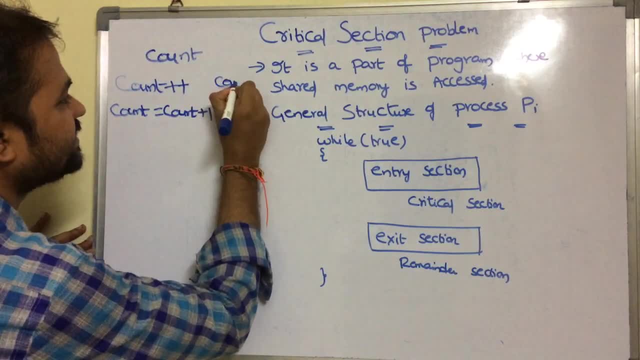 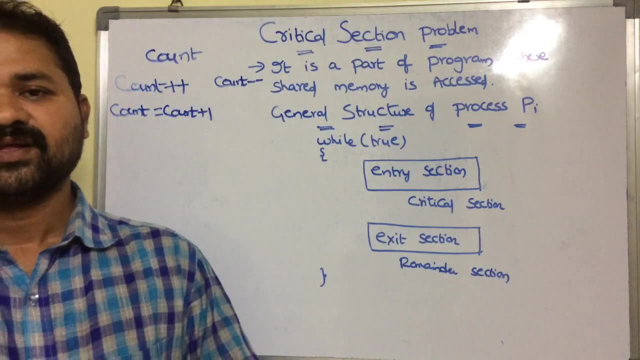 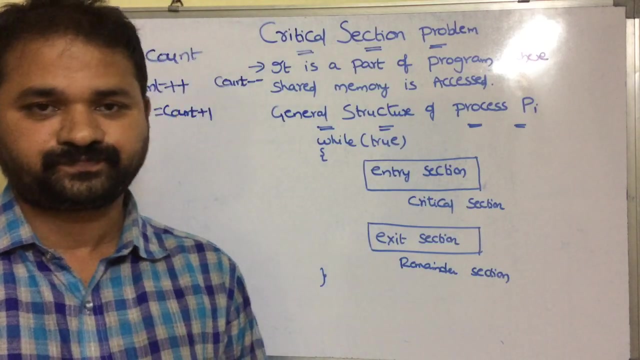 So we can write the statement as count minus minus. So this statement can also be written as: count is equal to count minus one. So in producer consumer problem, accessing count variable is nothing but critical section. So why it is denoted as critical section. 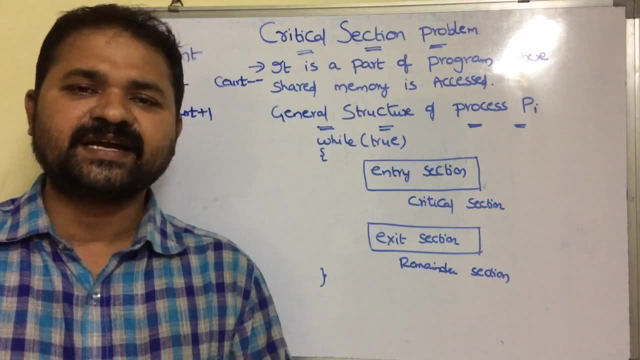 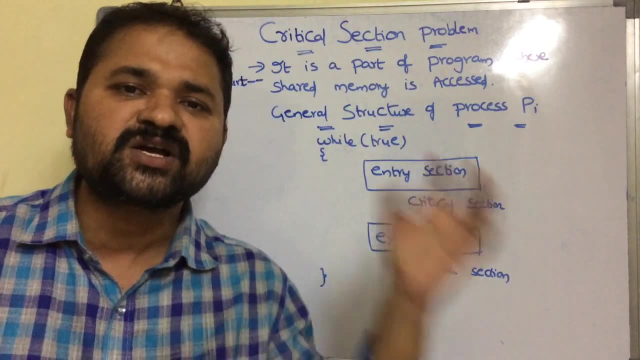 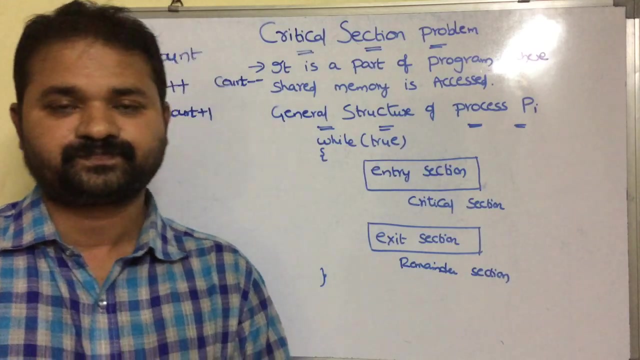 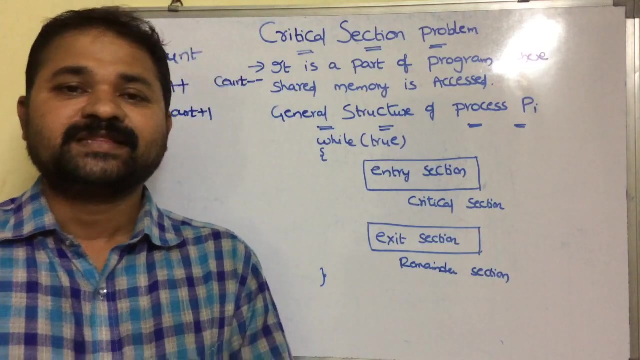 Why? because If producer process tries to access count variable, then consumer process should not access count variable. Here accessing count variable is nothing but a critical section. That means if producer process tries to access critical section, then consumer process is not allowed to access the critical section. 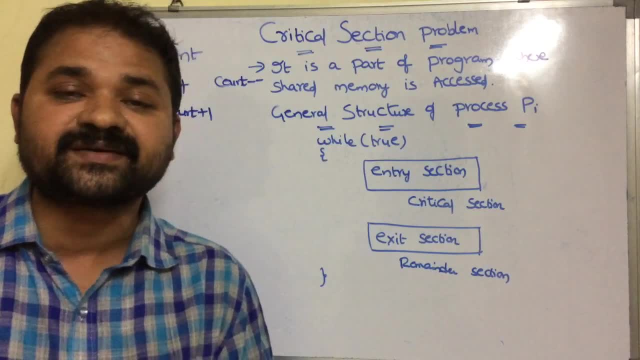 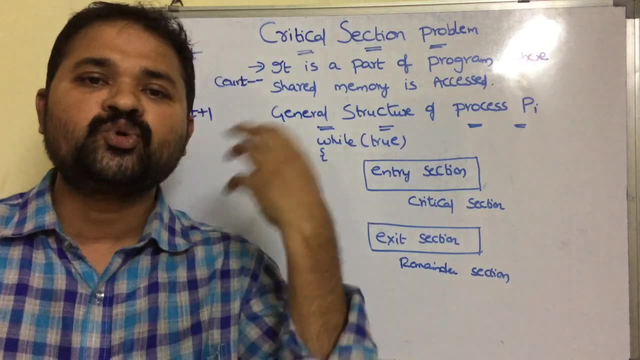 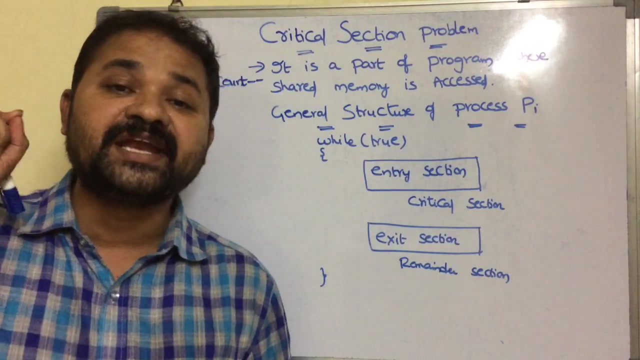 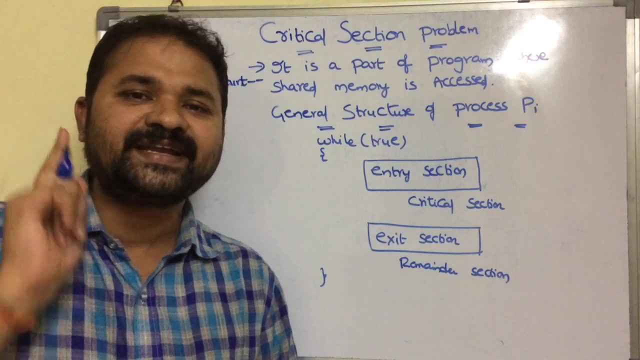 Likewise, when consumer process is trying to access critical section, then producer process is not allowed to access the critical section. So that means the accessing to the critical section must be mutual exclusive. That means the critical section should contains only one process at a time. 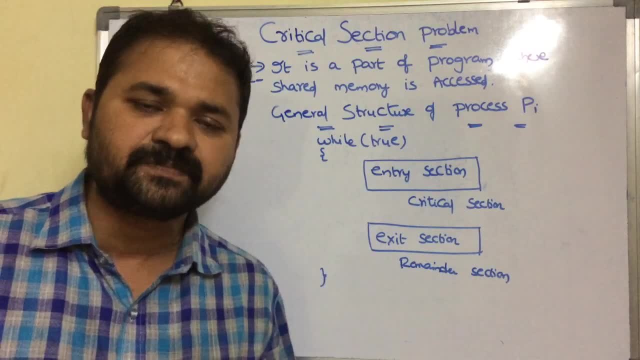 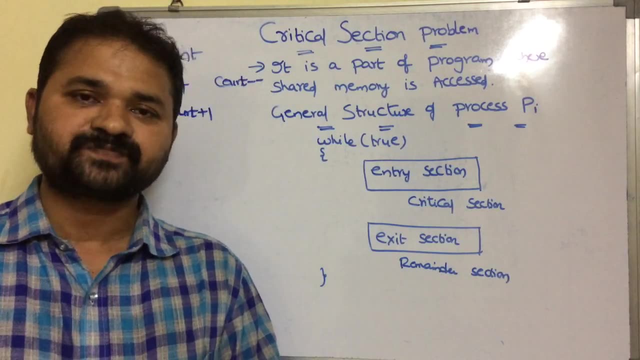 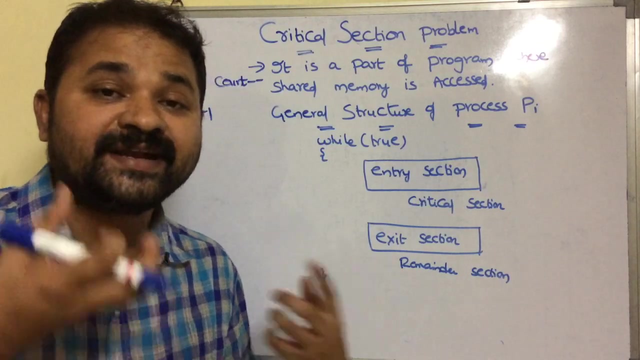 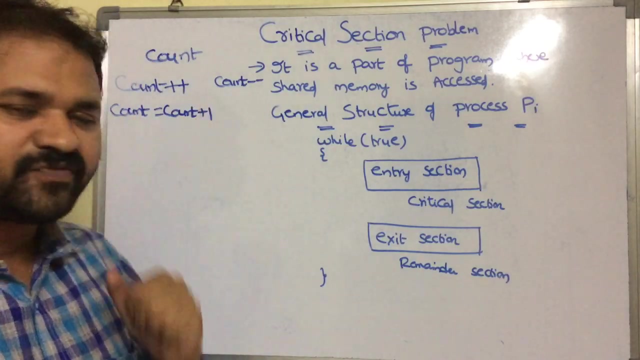 If producer process is in the critical section, then consumer process is not allowed to enter in the critical section. Likewise, when consumer process is in the critical section, then producer process is not allowed to enter in the critical section. If both producer and consumer process at a time access the count variable, then it produces wrong results. 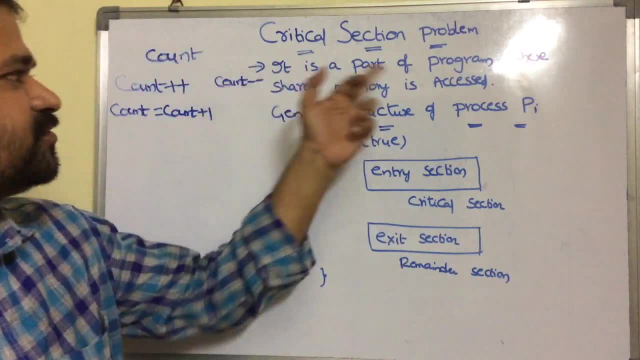 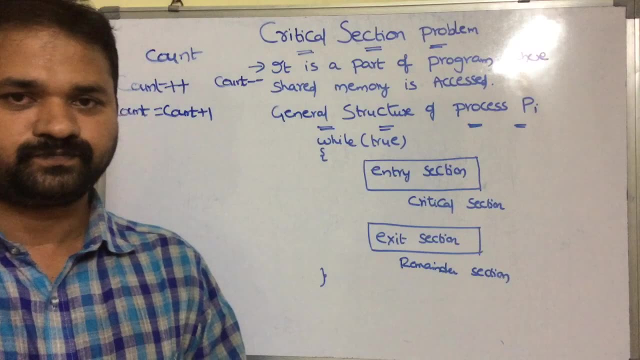 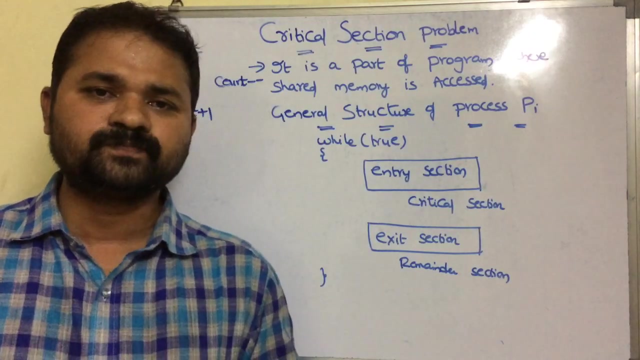 Okay, So in order to solve that problem only, we are using this problem- critical section problem. Okay, So this is about what is critical section. Next, how we can solve the critical section. In order to solve the critical section problem, we have two solutions. 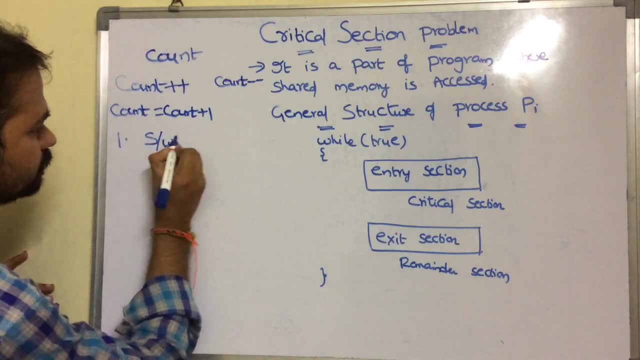 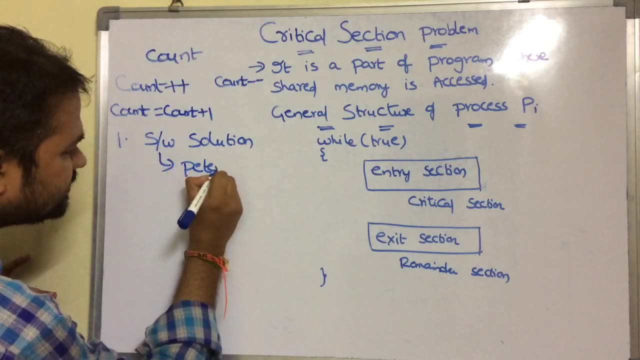 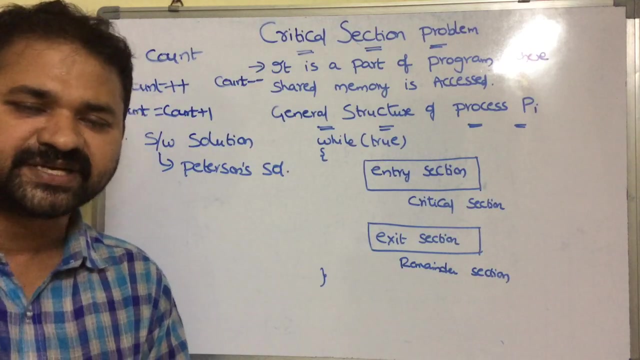 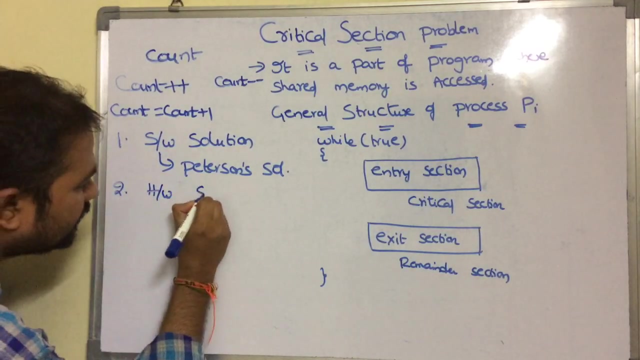 The first solution is a software solution. Here the software solution is nothing but Peterson solution. We will discuss about the software solution, such as Peterson solution, in the next video. And the second solution is hardware solution. Here the hardware solution is nothing but synchronization hardware. 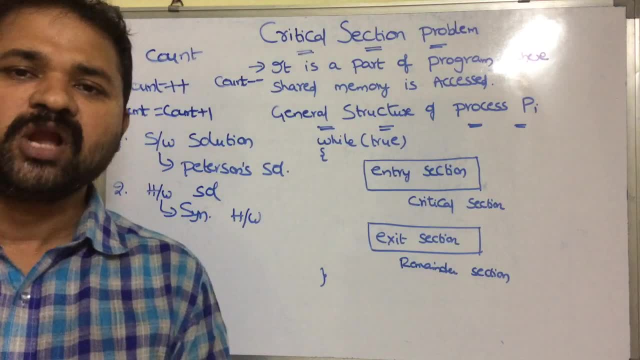 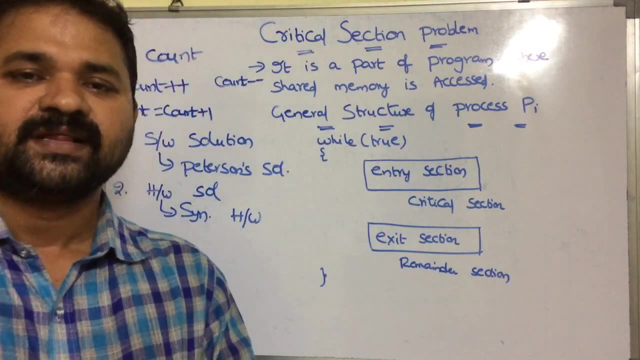 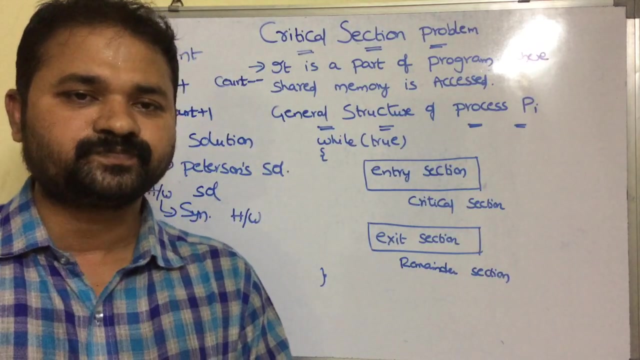 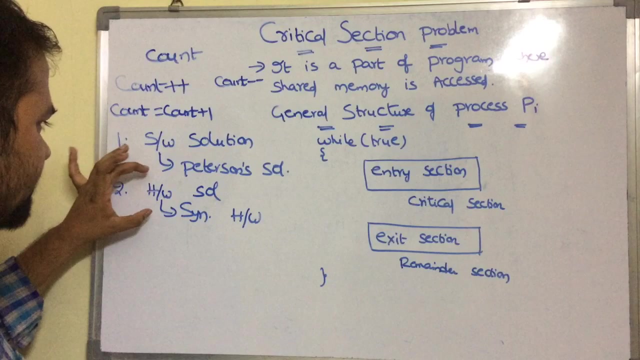 So we can solve the critical section problem in two ways. The first way is the software approach. The second way is hardware approach. Here the software approach is nothing but Peterson problem, Whereas the hardware solution is nothing but synchronization hardware. We will discuss about Peterson solution as well as synchronization hardware in the upcoming videos. And here the point is, any solution to the critical section problem needs to satisfy three requirements. It may be either Peterson solution or synchronization hardware. It has to satisfy three requirements. So let's see what are the three requirements which are to be satisfied in order to solve a critical section problem. 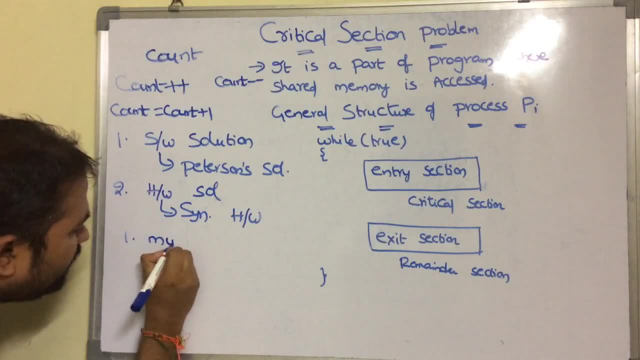 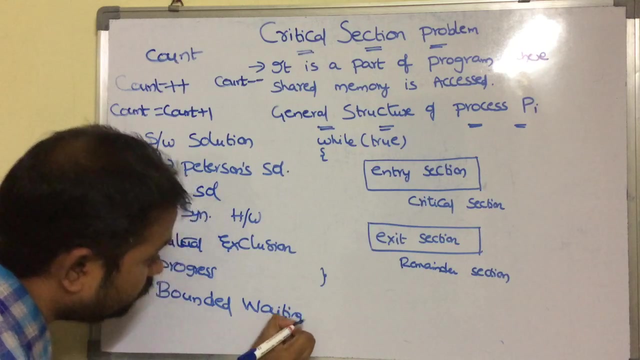 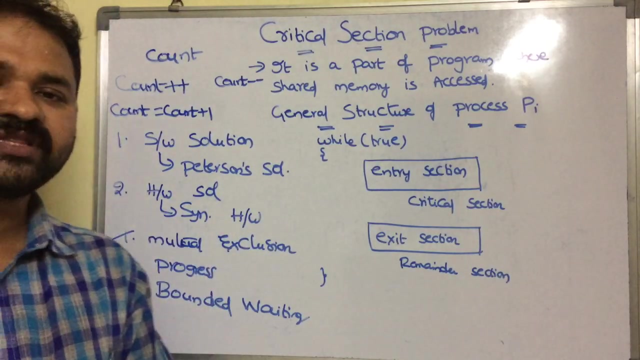 The first requirement is mutual exclusion. The first requirement is mutual exclusion, The second requirement is progress, Whereas the third requirement is bounded waiting, Bounded, waiting. So any solution to the critical section problem must satisfy these three requirements. So let's see about the first one, mutual exclusion. 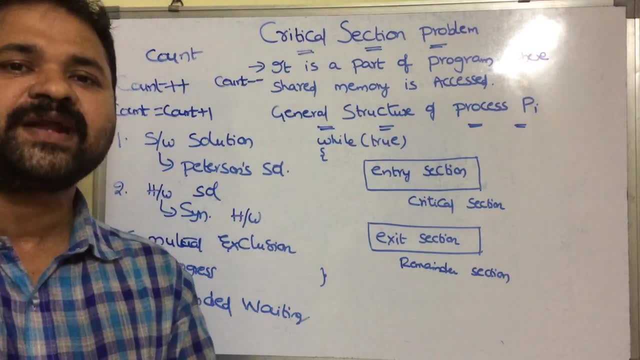 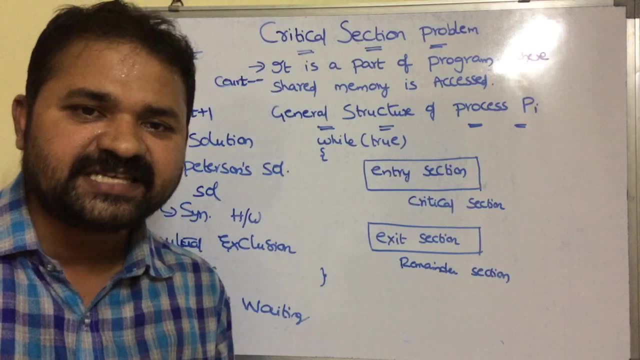 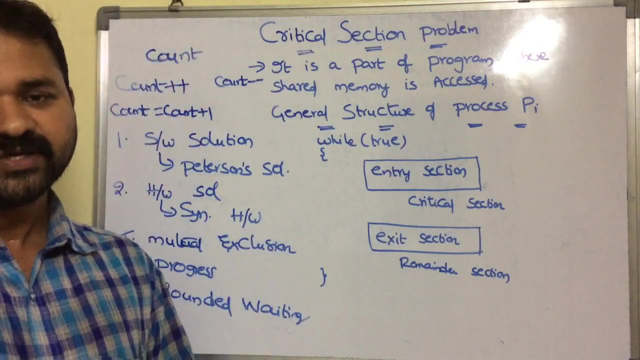 Mutual exclusion means at a time only one process is to be in the critical section. When one process is in the critical section, then other process should not be allowed to enter in the critical section. So only when the first process comes out from the critical section. 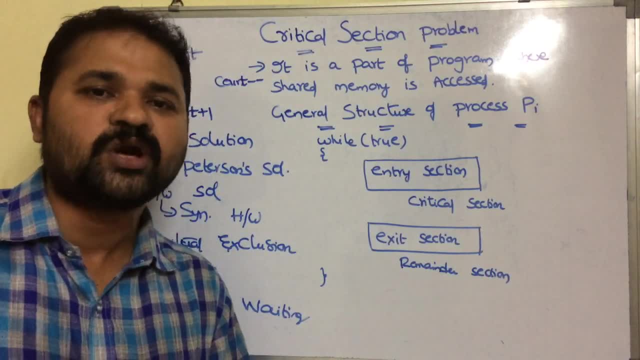 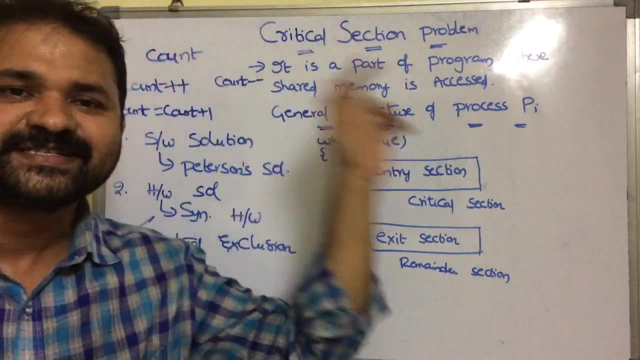 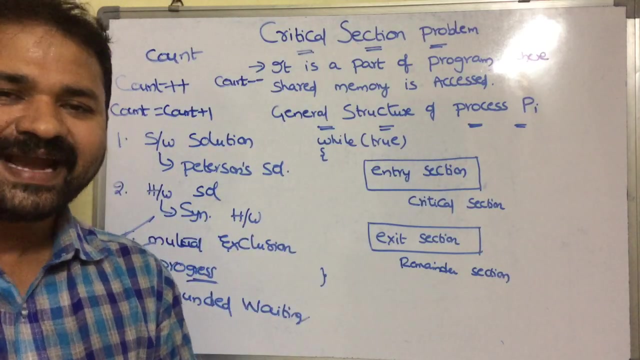 then only the second process is allowed to enter in the critical section. So we have to satisfy mutual exclusion in order to solve the critical section problem. Let's see the second requirement: Progress. So let's see what is a progress. Let critical section doesn't contains any process. 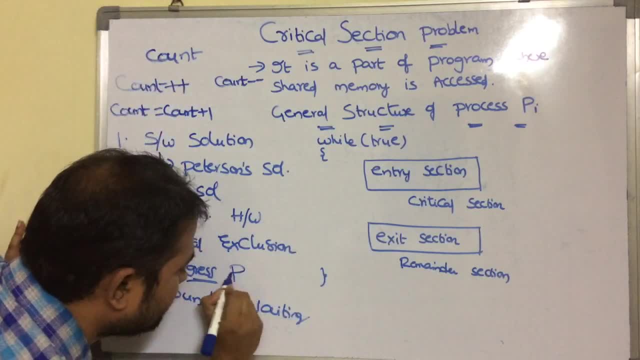 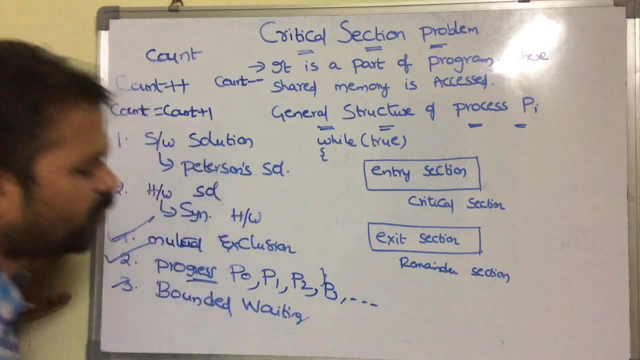 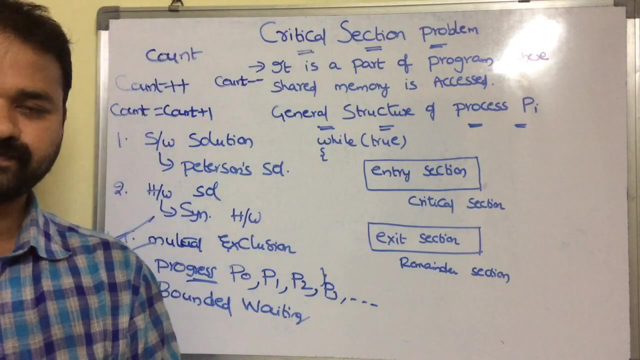 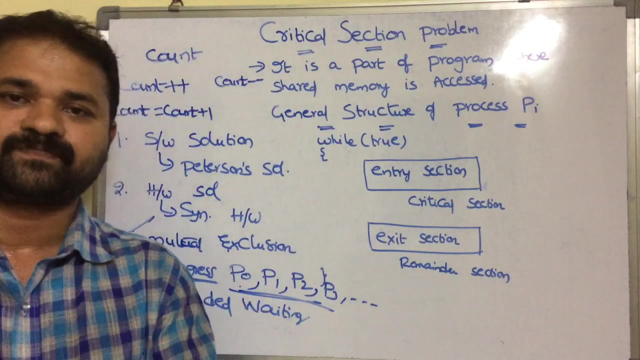 and a set of processes such as P0, P1, P1, P2, P3.. So, likewise, let we have several processes and all these processes are waiting for entering into the critical section. Then the decision about which process we enter into the critical section. 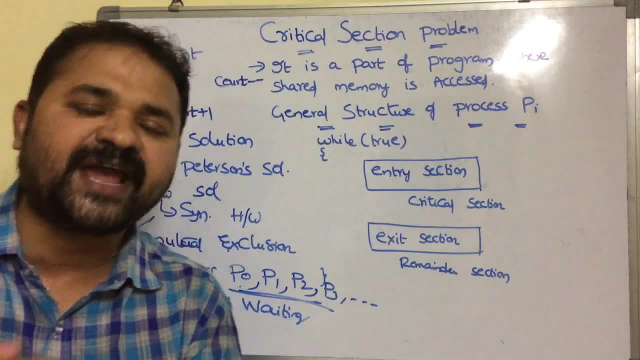 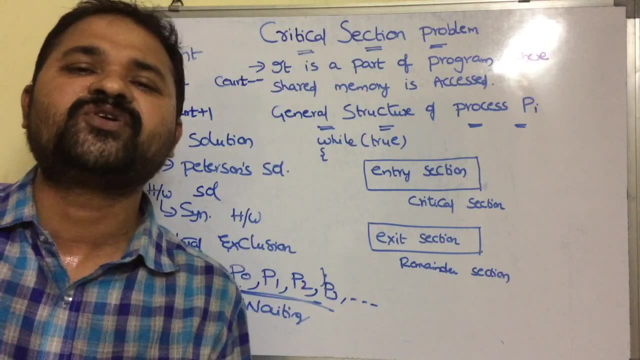 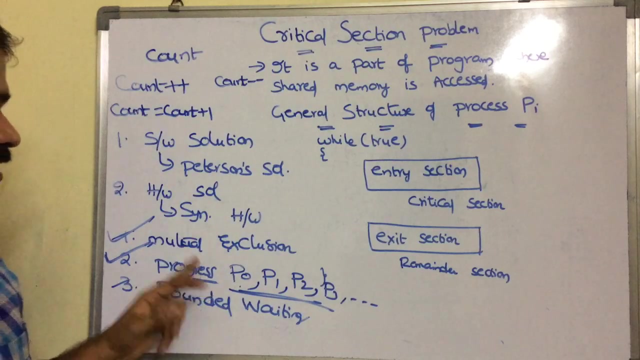 should be taken in a finite amount of time, So it should not be postponed for a longest period of time. indefinite amount of time. So that is nothing but the second requirement for solving a critical section problem. So what is the second requirement? Progress. 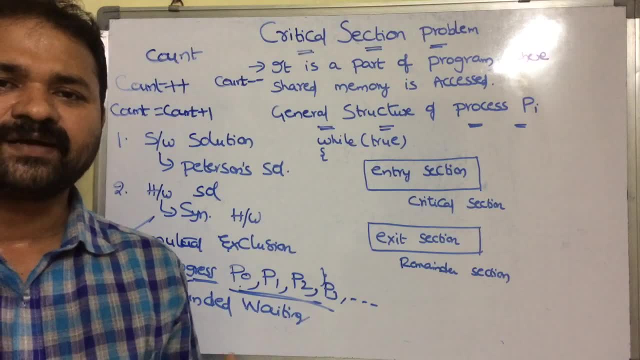 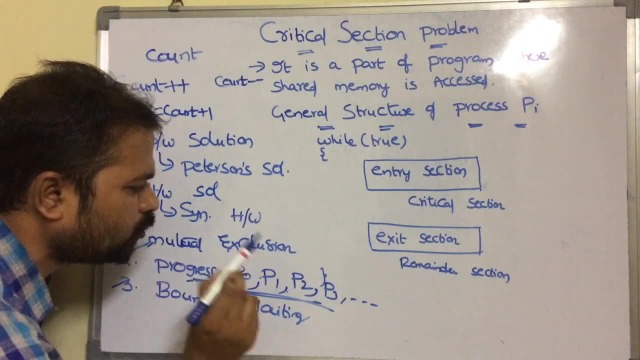 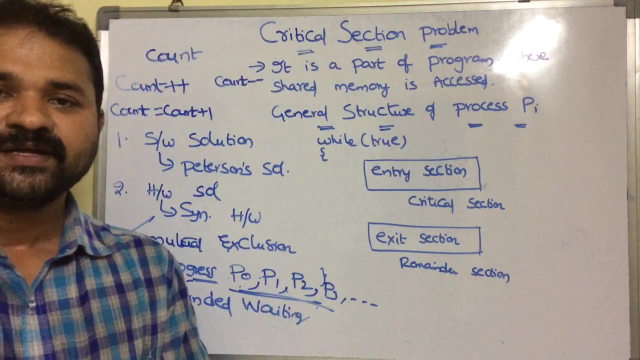 So what is a progress? Let us assume that the critical section is free and a set of processes such as P0, P1, P2, P3 etc. are interested to enter into the critical section. Then the decision about which process we enters into the critical section. 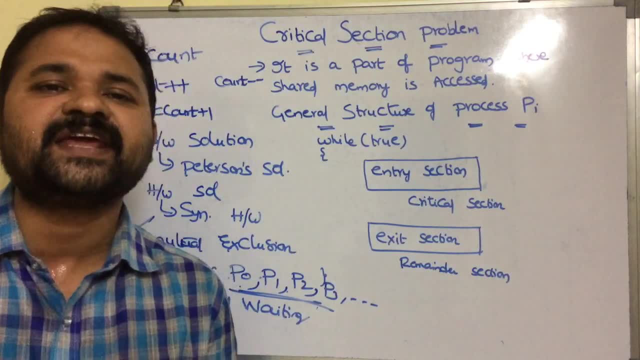 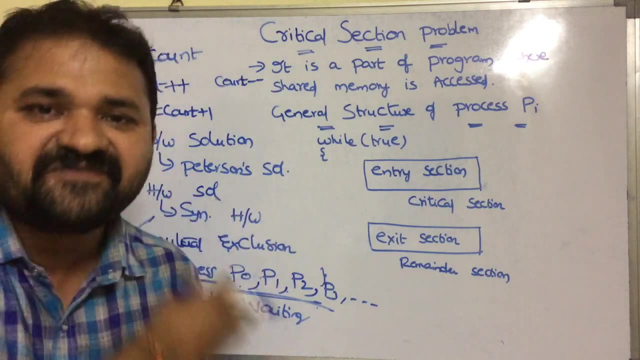 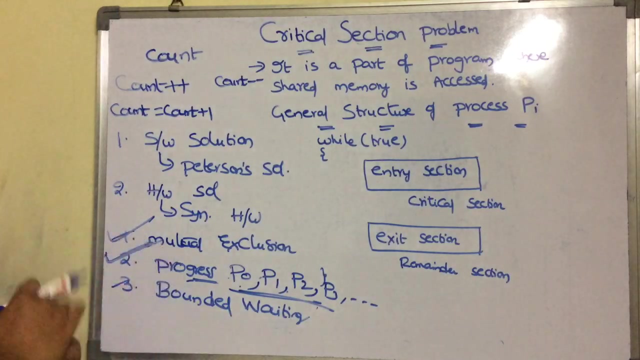 That decision should be taken in a finite amount of time. That decision should not be postponed for an infinite amount of time. That means there should be a progress. So that is nothing but progress. So now let us see the third one. So what is the third requirement? 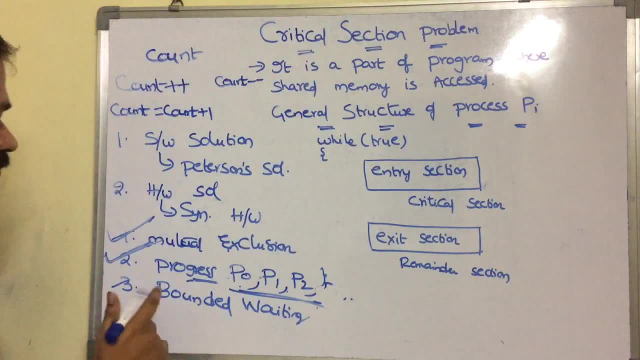 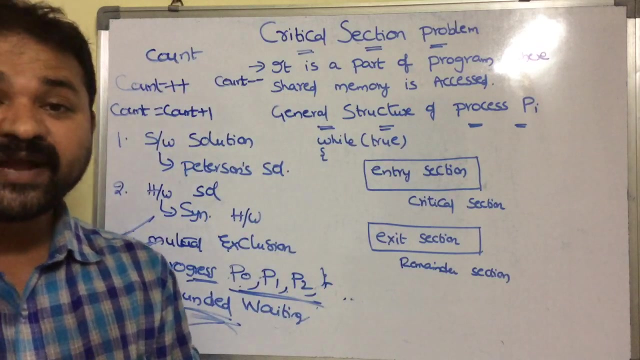 in order to solve the critical section problem: Bounded waiting. Here bounded means waiting. There should be a bound or limit on bounded means. here there are two types of buffers: Bounded buffer and unbounded buffer. So bounded means limited. The size of the buffer is fixed. 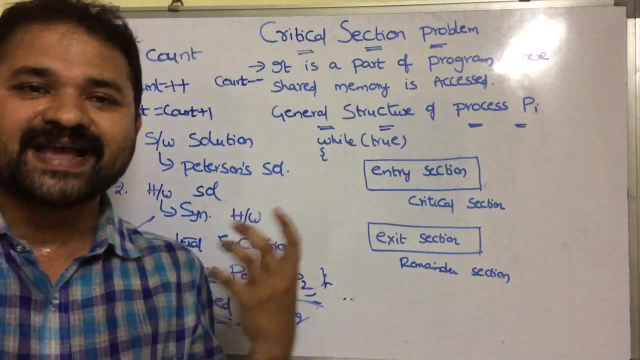 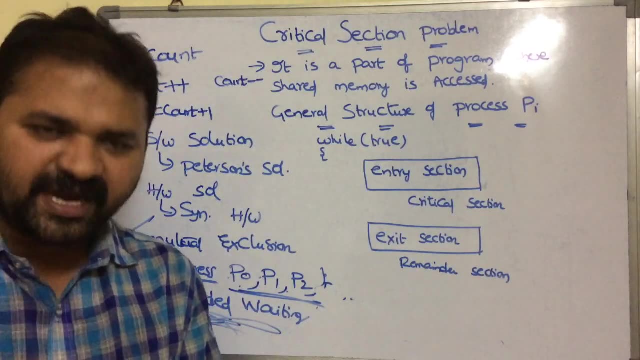 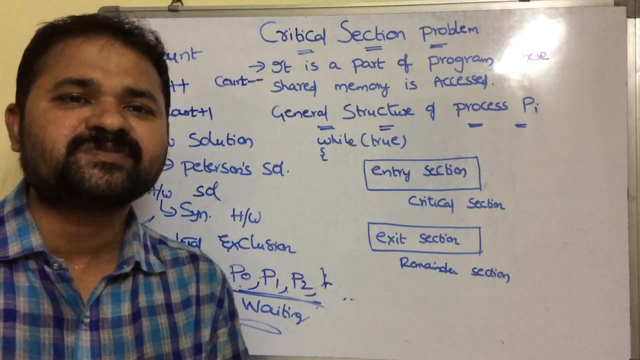 Whereas unbounded means the size of the buffer is infinite. So here, what is the third requirement? Bounded waiting. So bounded waiting means there should be a bound or a limit on the number of times a process can enter into the critical section When other process requires. 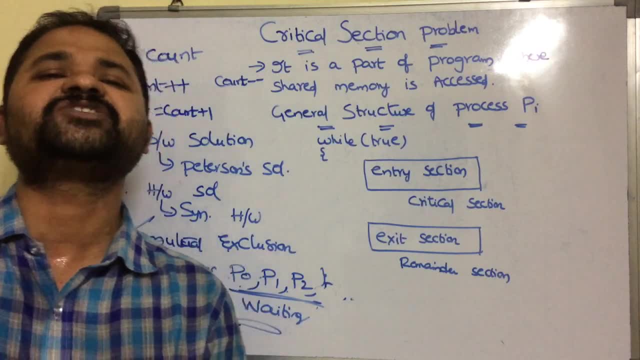 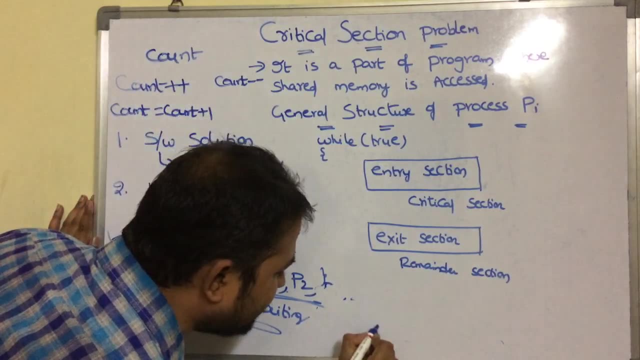 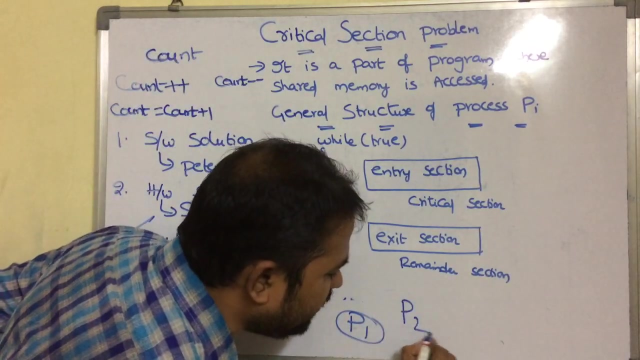 for entering into the critical section. Let us take an example Here. we have a critical section, So let it be the critical section. Let critical section contains P1 process And we have one more process called P2.. Let P1 is in the critical section. 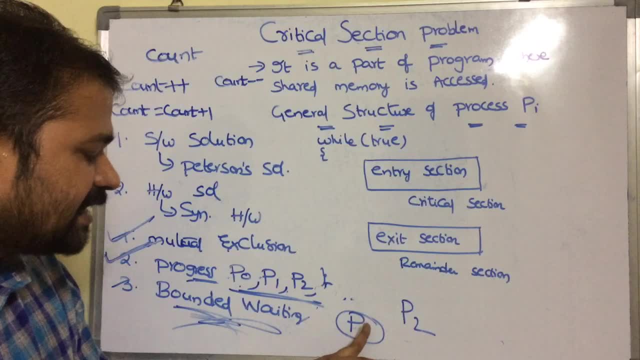 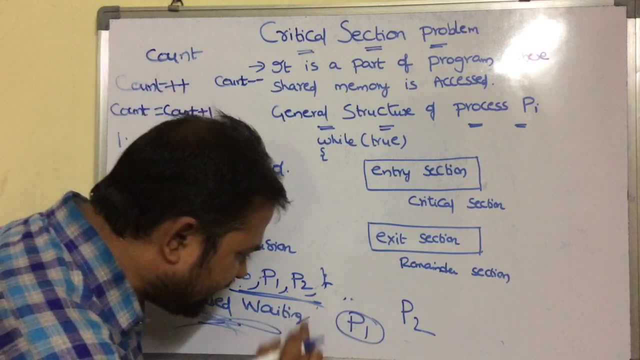 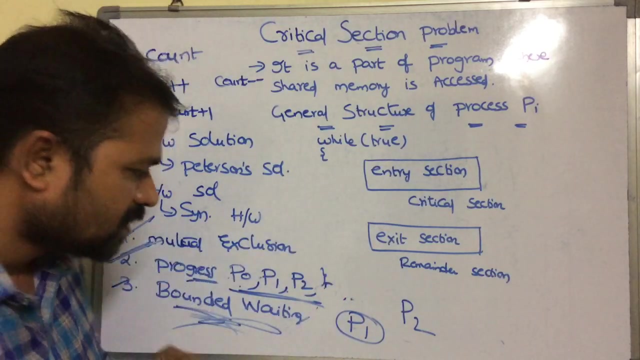 And P2 is waiting for entering into the critical section. But a critical section should contain only one process. So here critical section contains P1. So assumes that P1 process completed its execution. So P1 comes out of the critical section. So P1 comes out of the critical section. 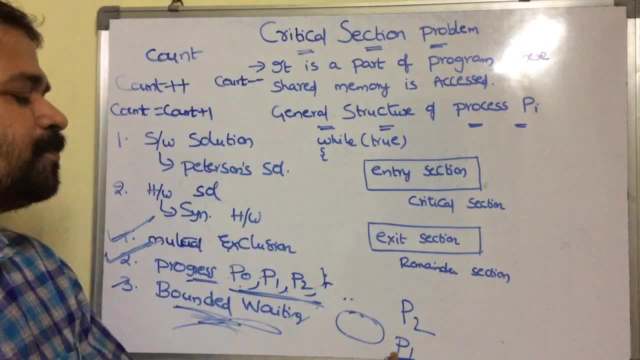 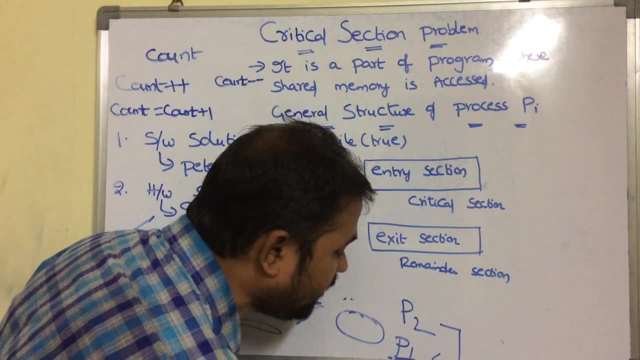 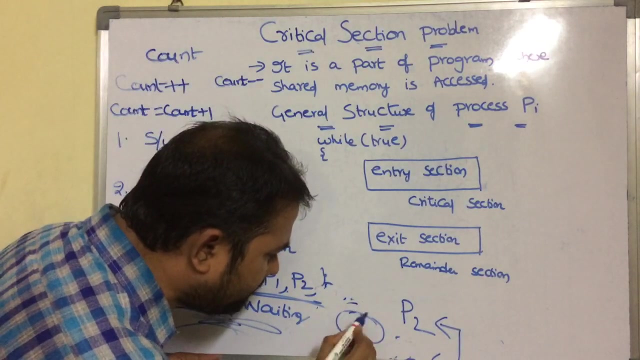 Let us assume that here P1 also put a request for entering into the critical section. So here there is a commutation between P1 and P2.. Let us assume that P1 entered into the critical section. So one more time: P1 entered into the critical section. 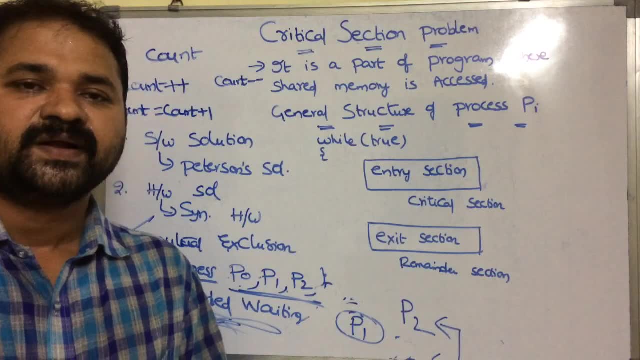 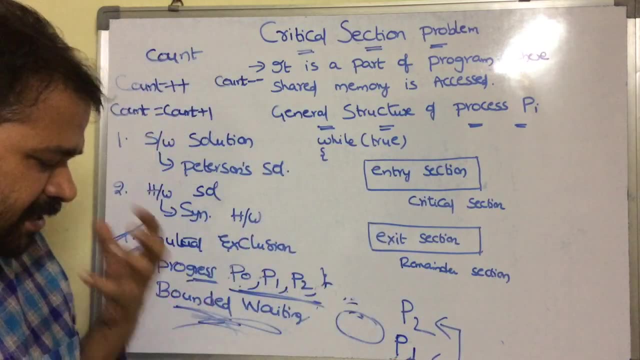 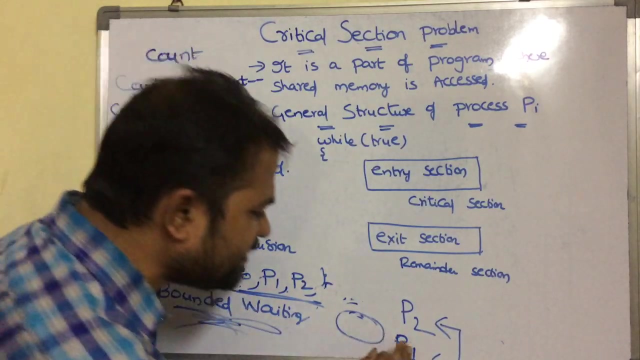 So let P1 completed all its operations. So P1 comes out from the critical section. So P1 comes out from the critical section. Now we assume that P1 puts one more request to enter into the critical section. Let us assume that operating system. 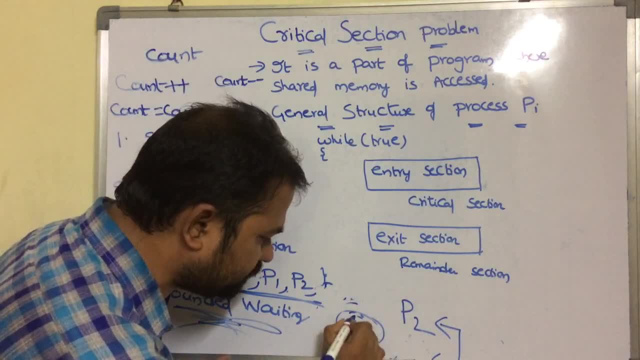 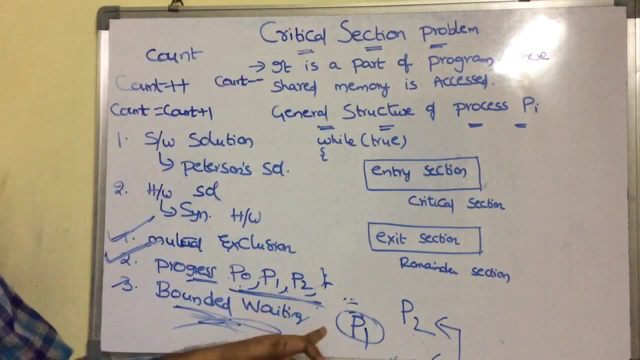 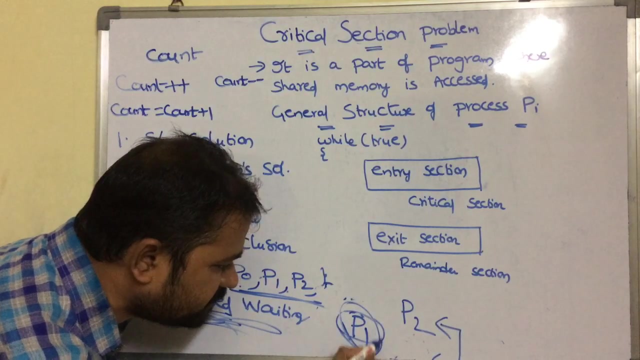 has given a chance for P1 to enter into the critical section. So here what is happening? P2 is waiting for too much time, amount of time. So here the point is bounded: waiting means there should be a bound or limit on a number of times. 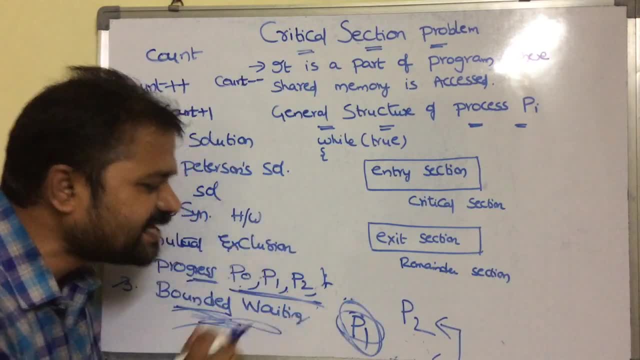 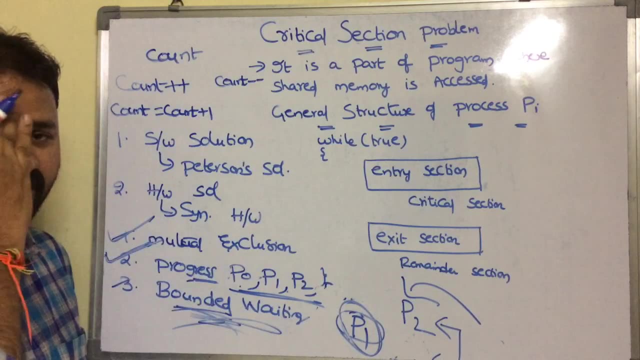 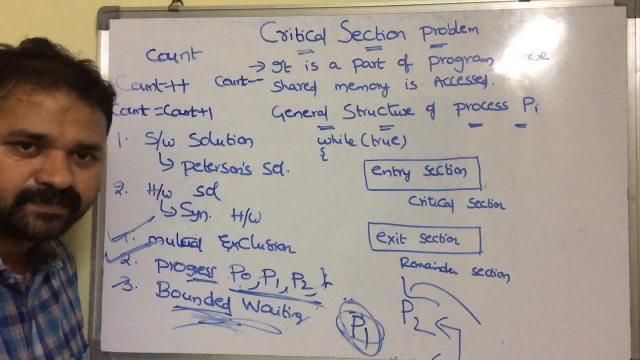 a process has to be entered into the critical section when other process puts a request to enter into the critical section. So here P2 puts a request to enter into to enter into the critical section, But P1 entered into the critical section. But here we have given. 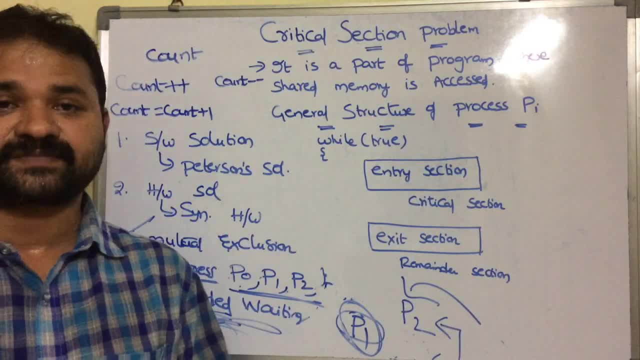 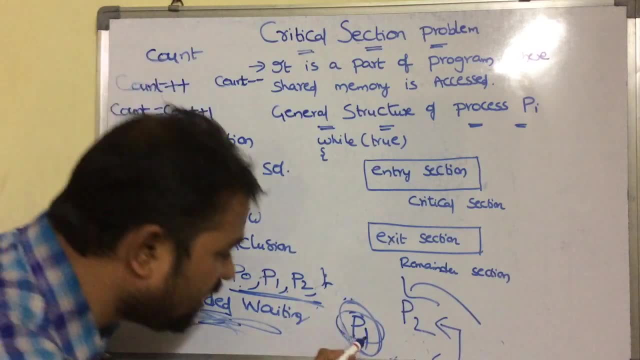 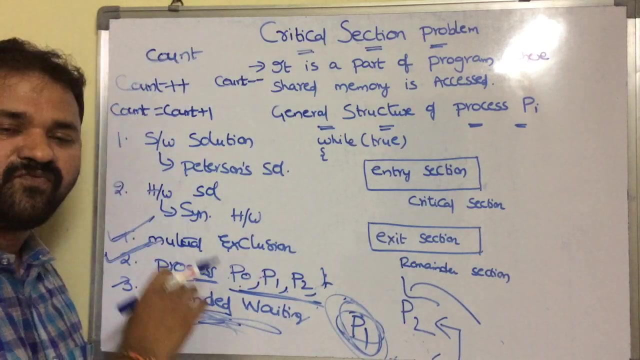 the process P1. so many chances to enter into the critical section. So here there should be a limit on P1 to enter into the critical section. So it has to be entered into the critical section for a bounded for a limited number of times. 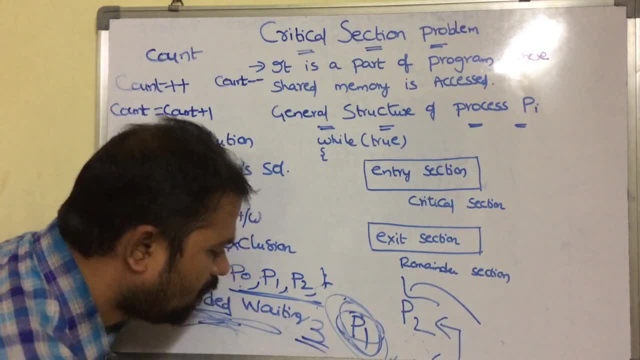 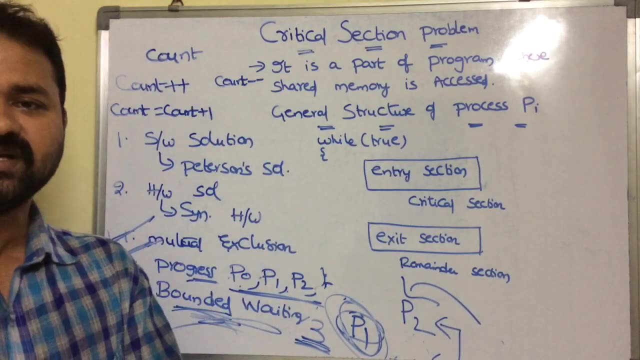 So let us assume that here the limit is given for three times, So that P1 has to be entered into the critical section for only three times. After that we have to given the chance for P2.. So that is nothing but bounded waiting. 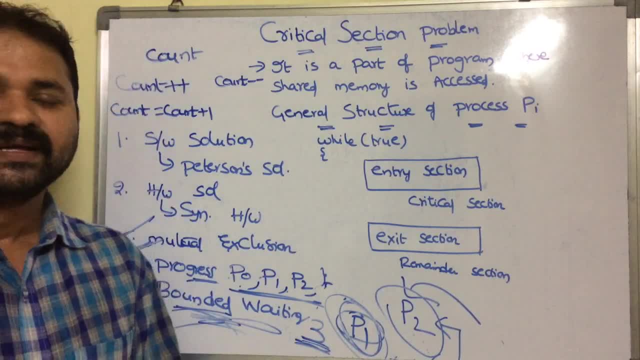 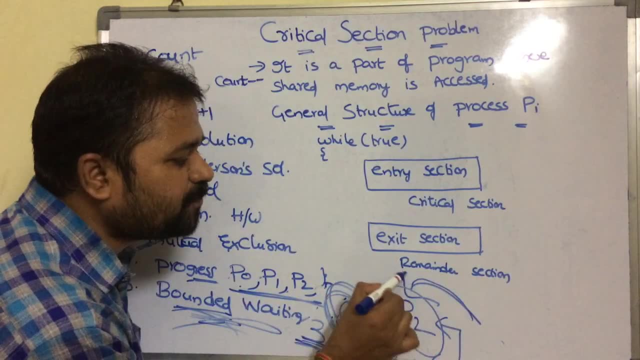 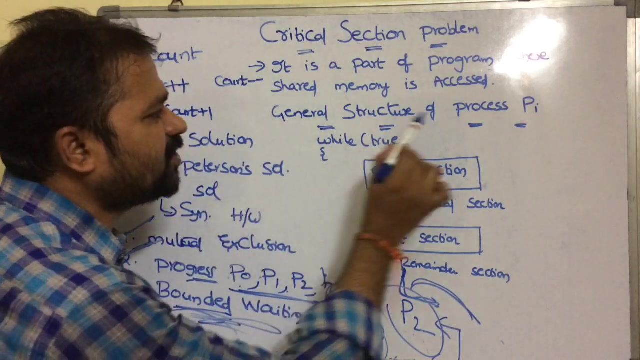 So there should be a bound or limit on the number of times a process can enter into the critical section when other process puts a request to enter into the critical section. Now let us see about general structure of a process P1.. So here, if any process contains: 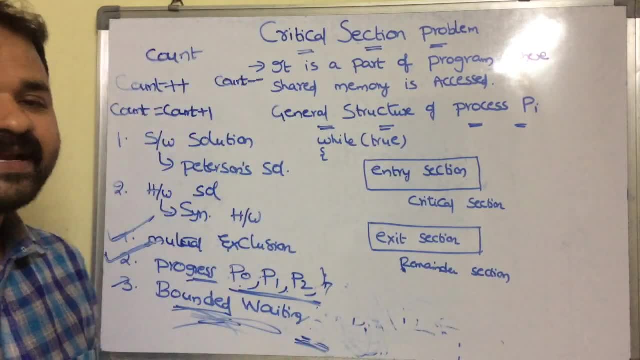 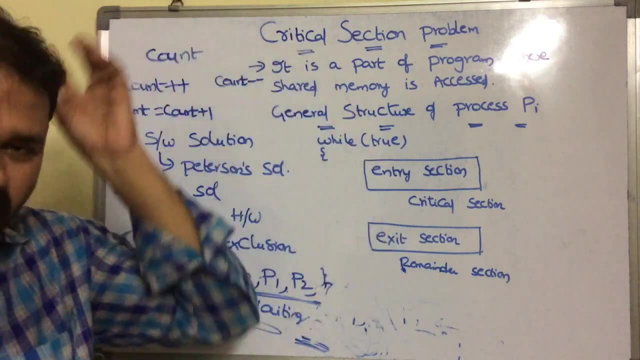 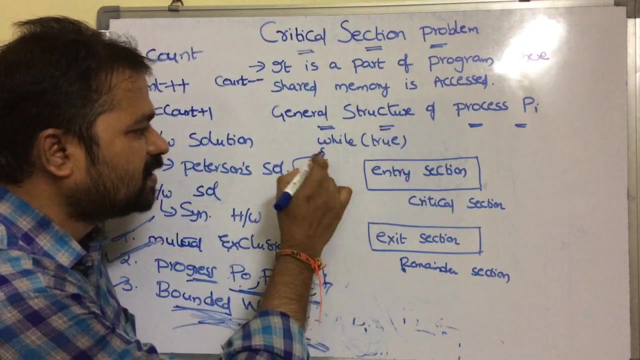 a critical section. So what is a critical section? A critical section is a part of the program which acts as shared variable. Then that process is divided into three parts. So this is nothing but while of true. So within the while loop, we have written the body. 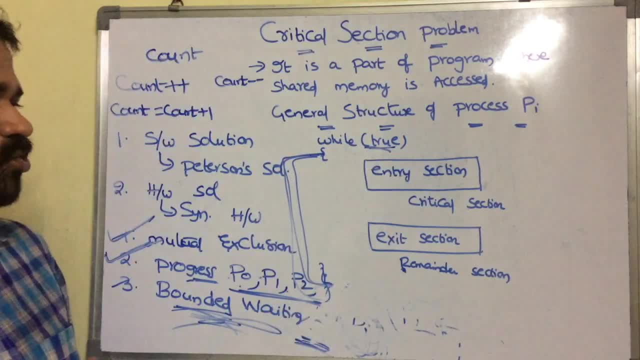 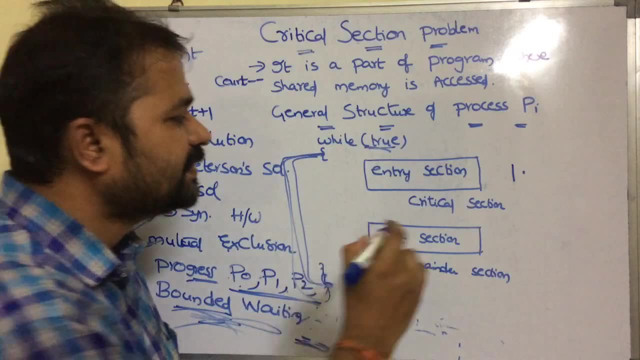 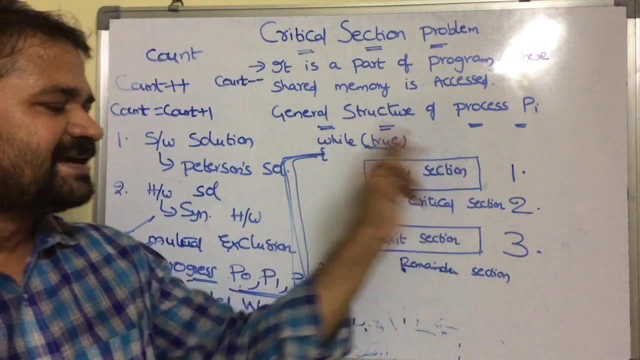 True specifies that this body is always executed Here. the process is divided into mainly three parts. The first part is entry section. The second part is critical section. The third part is exit section. So let us see the first one, Entry section. 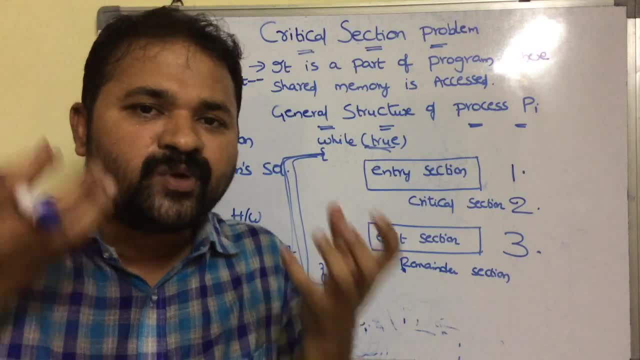 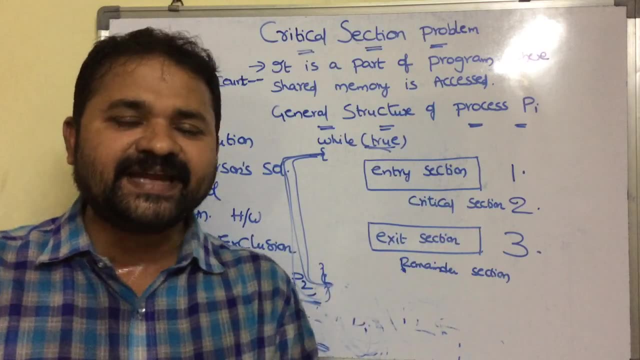 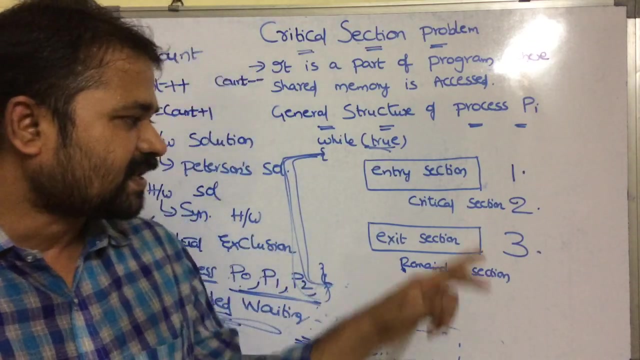 So whenever a process wants to enter into the critical section. So first it has to check whether the critical section contains some other process or free, Suppose if the critical section is free, Then the corresponding process will enters into the critical section. Suppose if the critical section 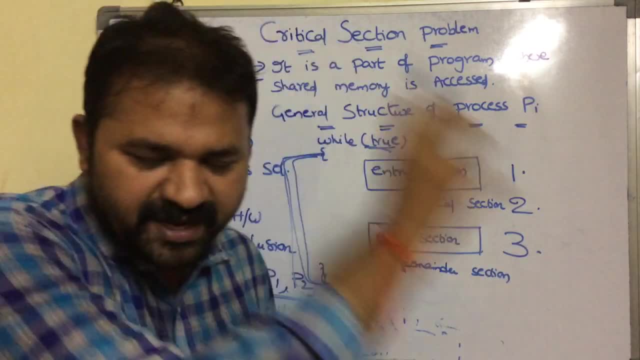 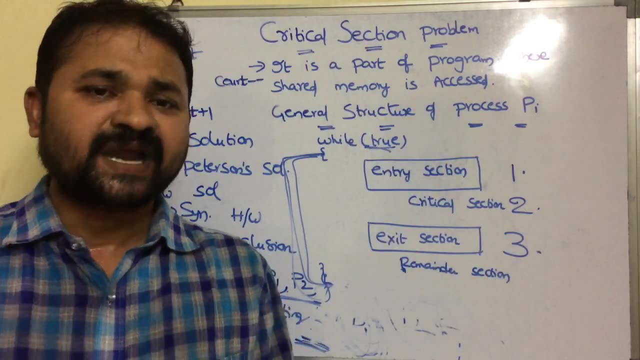 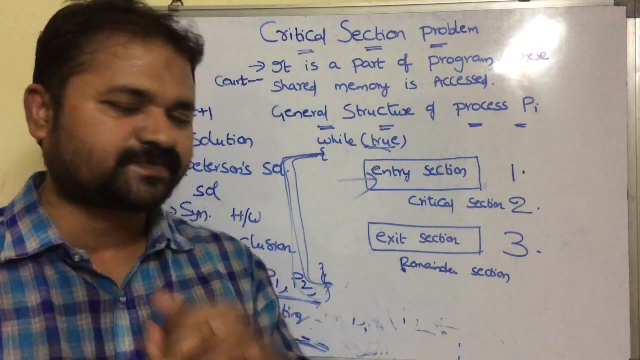 is already occupied, Then the corresponding process has to be. wait until that process comes out from the critical section So that corresponding code should be written in entry section. So entry section contains a code, whether that process is entered into the critical section or not. 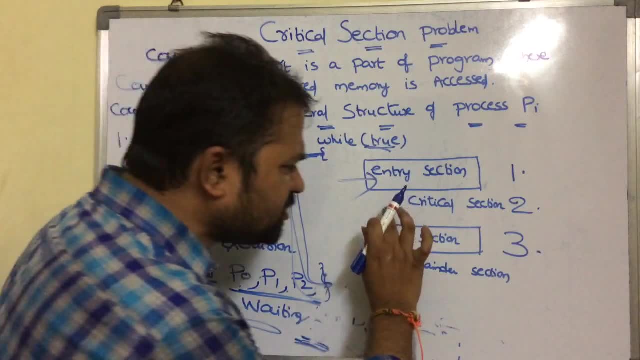 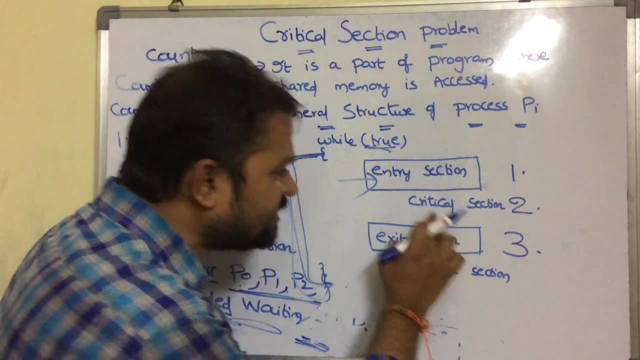 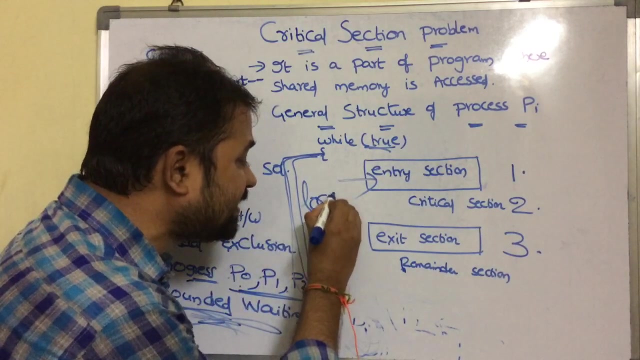 Let us assume that here the critical section is free, So the corresponding process can enter into the critical section. Before entering into the critical section, the corresponding process locks the critical section. That means wherever that process comes out from the critical section, then only some other process. 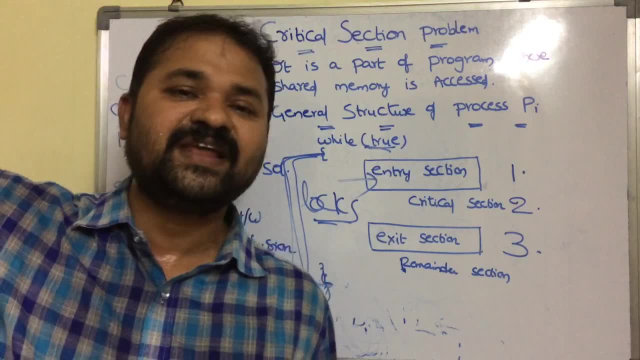 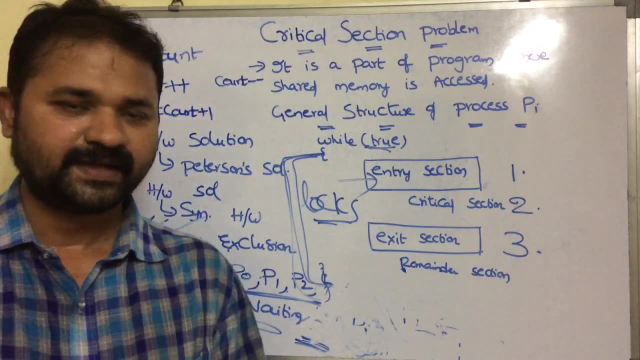 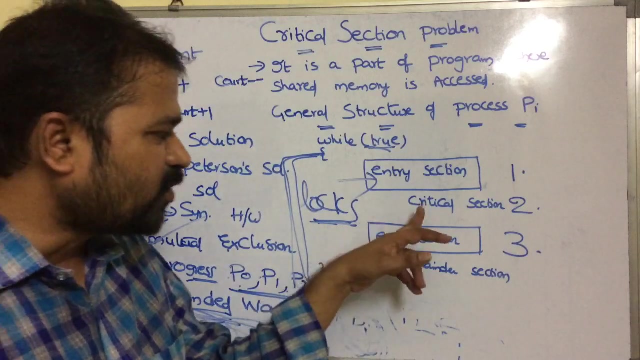 will be entered into the critical section. Some other process will be allowed to enter into the critical section. Why? because here we have to satisfy mutual exclusion. Okay, So let us assume that critical section is free, So that the first process enters into the critical section. 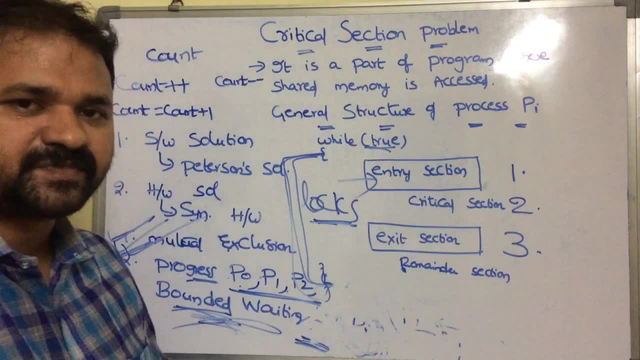 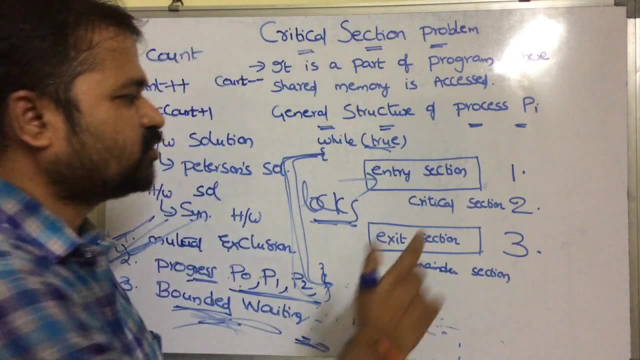 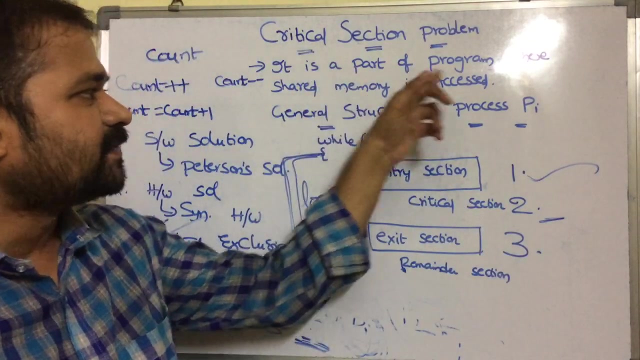 Before that, the first process locks the critical section So that no other process should be allowed to enter into the critical section. So this is the first part. The second part is critical section. So what is a critical section? It contains a part of the program. 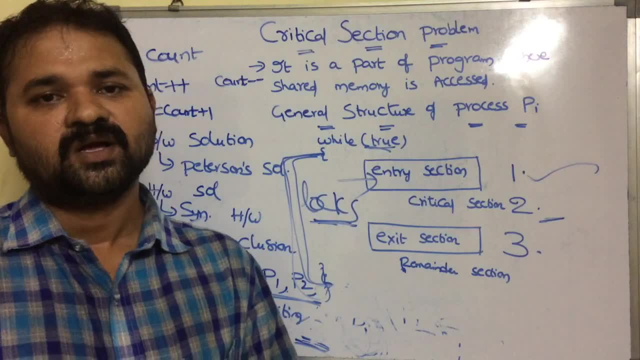 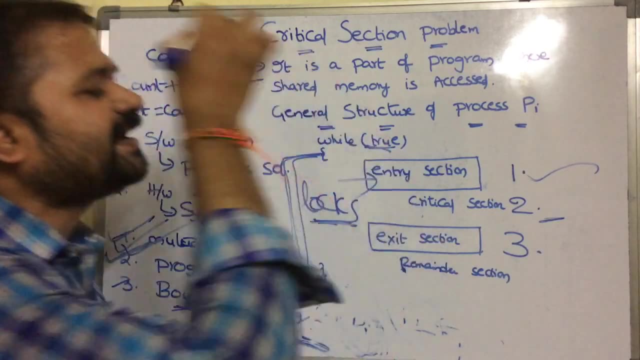 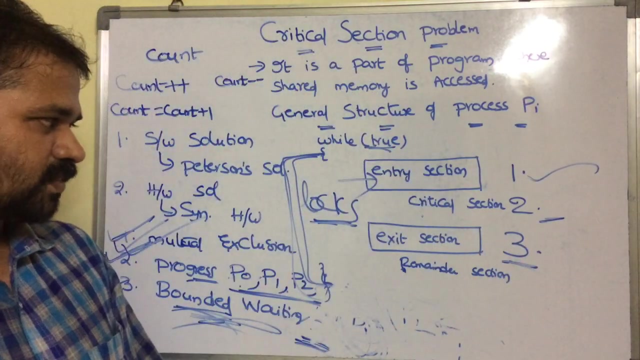 where the shade variable is to be accessed. So the corresponding process will execute in critical section and after that it comes out from the critical section. So whenever it comes out from the critical section then we have to execute exit section In entry section. we lock out the critical section. 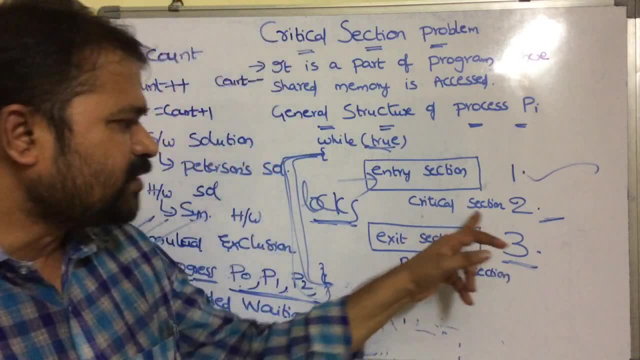 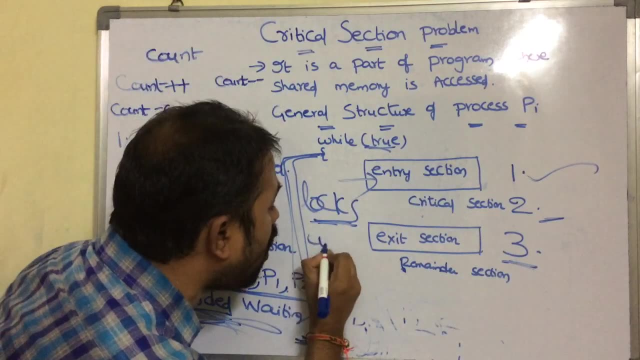 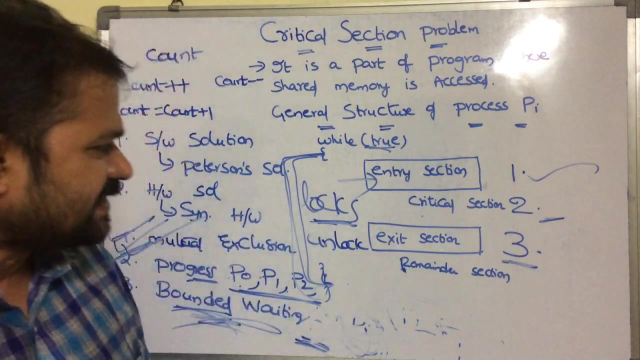 So that no other process should be allowed to enter into the critical section, Whereas in exit section we have to unlock the critical section. We have to unlock the critical section So that it specifies that the critical section is free, So that other processes which are waiting. 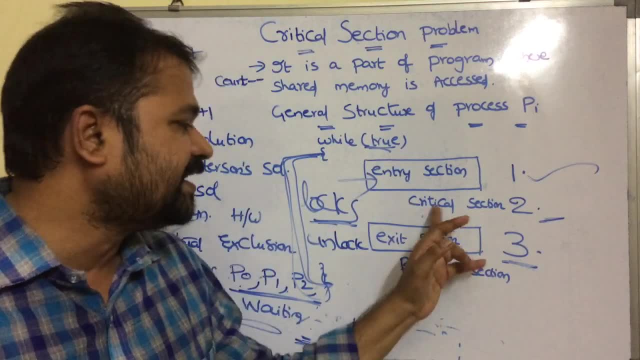 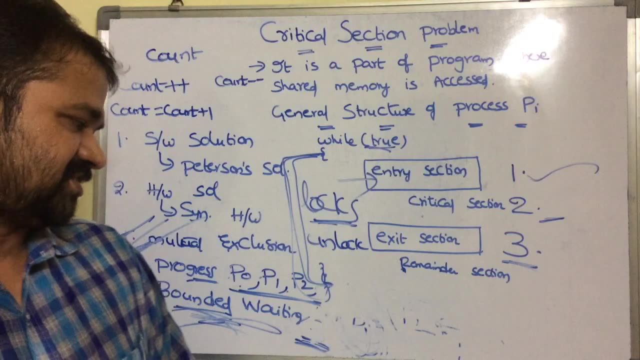 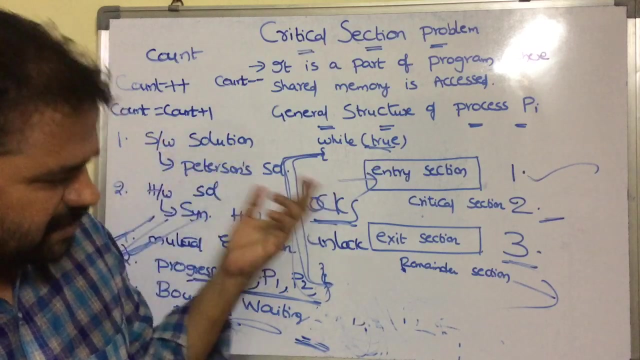 to enter into the critical section are allowed to enter into the critical section. So exit section mainly contains the code which unlocks the critical section And this is the optional one, reminder section. So reminder section means it doesn't belong to the entry section. critical section as well as exit section.